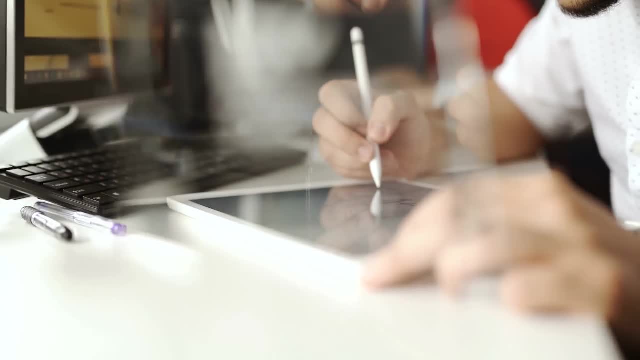 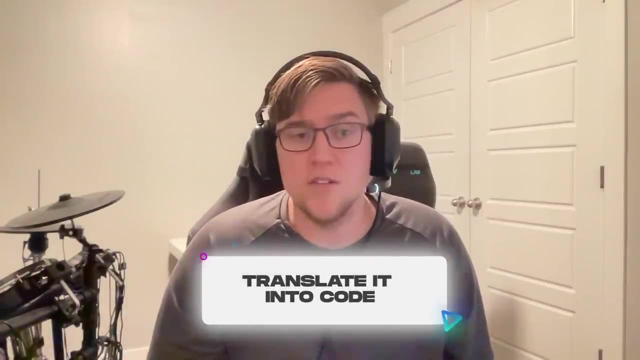 an image or a Figma file or you know something in Sketch. Your job is just to translate it into code. So I mean you'll need to know CSS. I mean, I'm just going to plug one of my favorite tools. 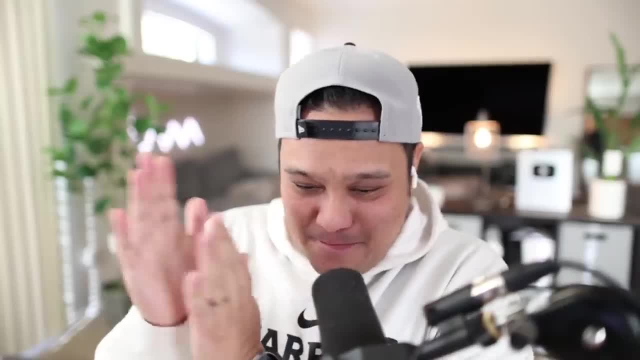 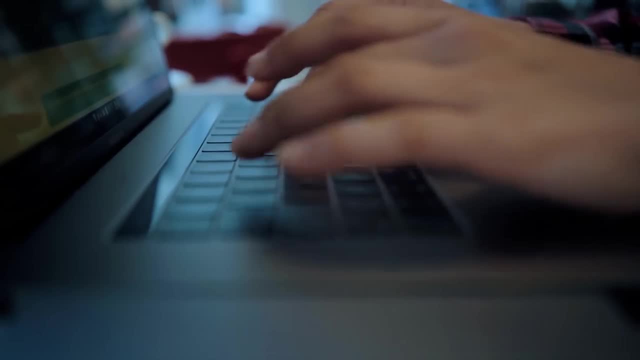 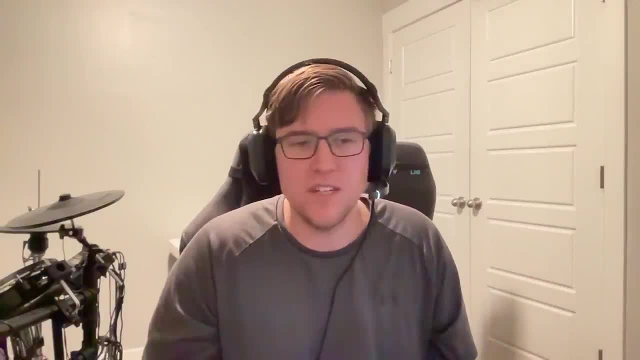 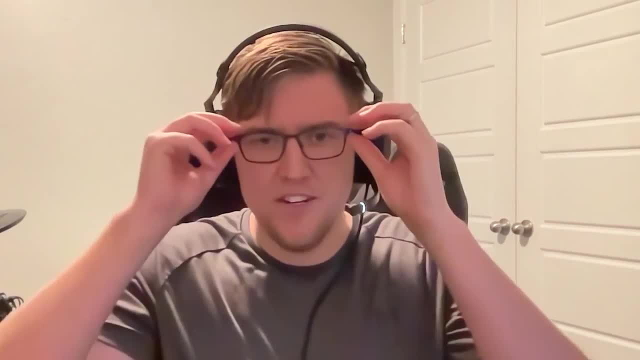 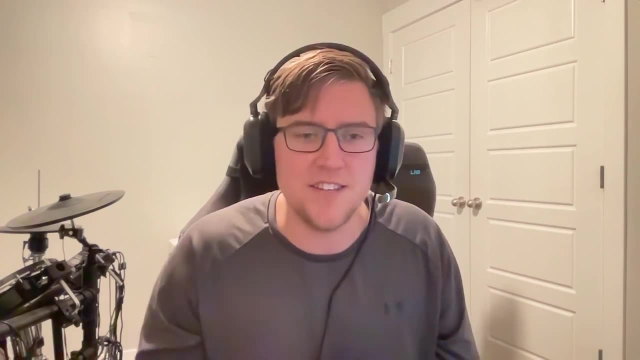 when you get stuck. But what is hard is writing like clean CSS. So like I think we're all familiar with the idea of clean code, things like you know, not reusing code, You kind of abstract into functions, Writing clean CSS is, like I'm convinced, a near impossibility. So the answer: is you do need to learn HTML and CSS, but you're going to need to spend much more time on JavaScript, Like my guess is, 75% plus of your learning journey to that first front-end job is going to be JavaScript in some framework. I- 1 million percent, 100% agree with what Lane just said. Okay Now. 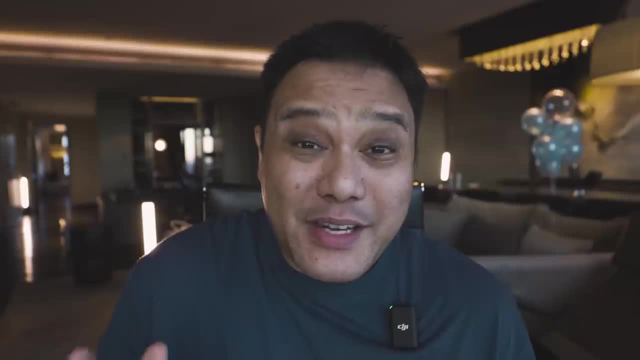 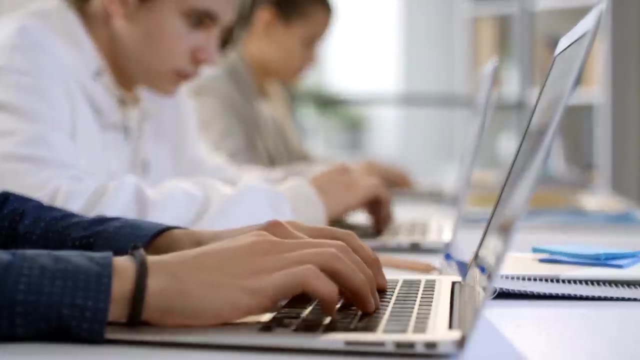 this is a very important topic And so listen carefully. So I think one of the biggest mistakes that an aspiring developer makes when learning how to code is that they spend way too much time either learning particular languages, spending way too much time that they need to, or again. 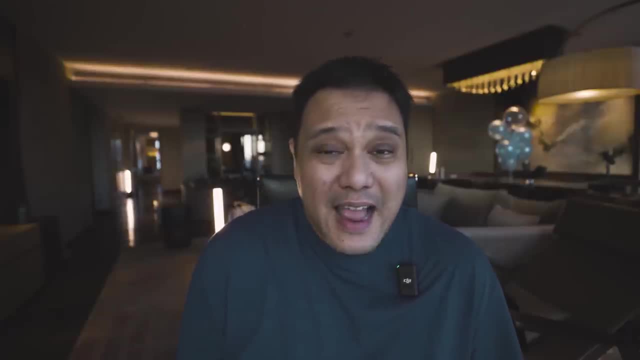 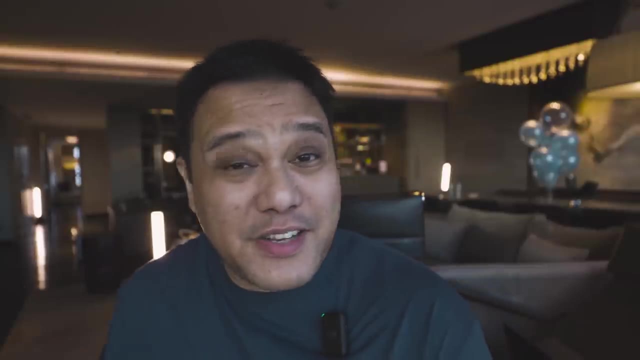 just to add on top of that, learning the wrong technical languages out there. right, And just like what Lane said, what people tend to do is spend way too much time on HTML CSS. Why? He said that when you work as a front-end developer, a lot of aspiring developers think that you need to be. 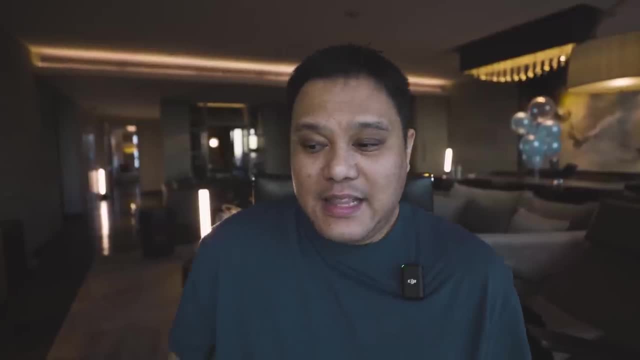 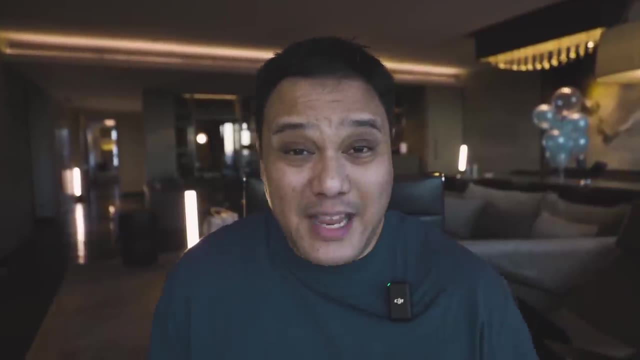 the best designer. A lot of aspiring developers think that you need to have good design skills. No, that is not the job of a front-end engineer. front-end developer, web developer, front-end software engineer- you name it. Our job is to take a design that a UI UX designer gives us. 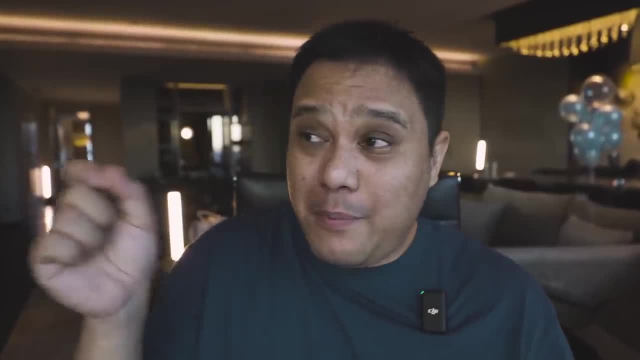 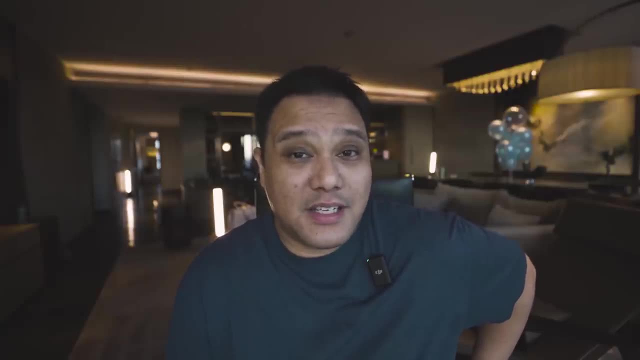 And when we turn that design into reality, we don't have a pen and paper, but using actual code. And so I like the point that he said, because what Lane said was people spend way too much on HTML CSS, People spend way too much on 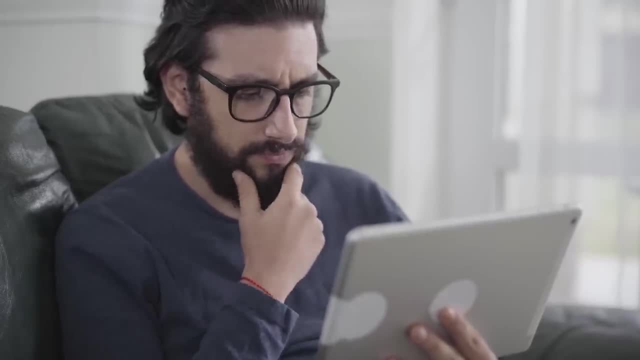 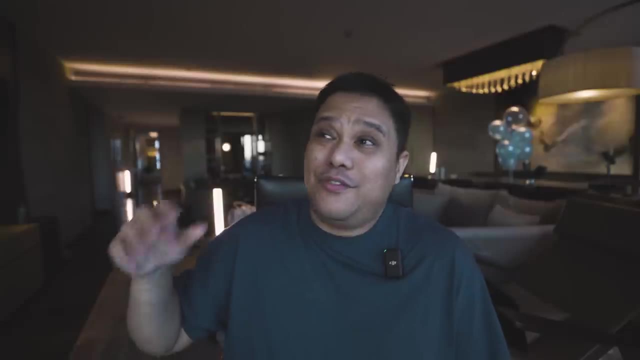 that thinking that they have to be the ones who think of creative designs. But the thing is, that's not our job at all. Our job is to turn what people created with Photoshop, with Adobe XD, with I don't know you name it. They create these beautiful designs and our job is to turn. 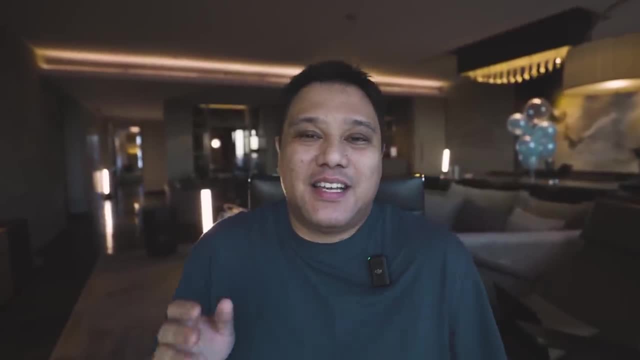 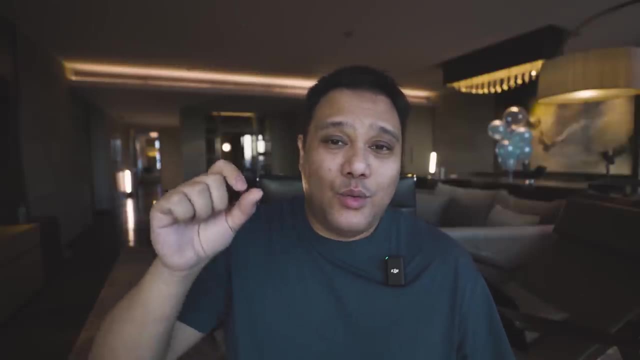 that into an actual picture and code. So then, how much HTML and CSS does a developer even need to have to get hired? What you need to know is pretty much how to what. What is the DOM right? What is the basic structures when building a website using HTML? I mean, look at Craigslist. 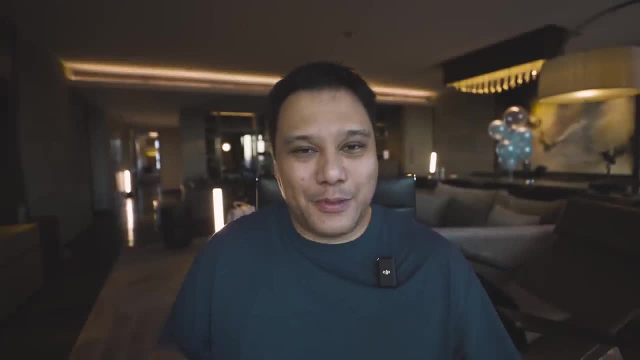 They have all of the basics down on craigslistcom. Not the best example, but that's literally HTML. Maybe some CSS to make the website more mobile friendly, but that's pretty much it, plain and simple. I think that what you need to do is just know what devs are, what labels are right, What 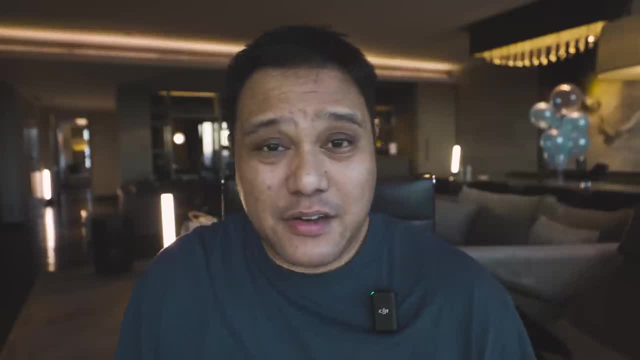 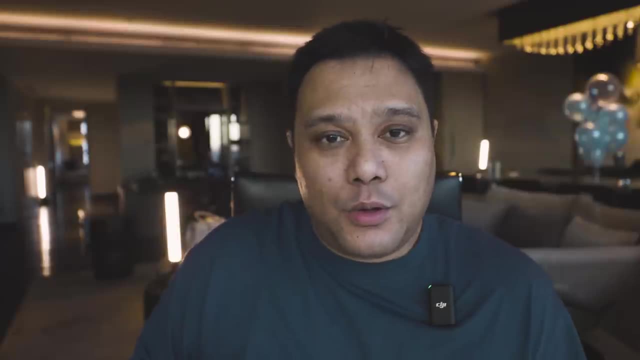 is the header? What is the body? What are the HTML tags? What is the anchor tag? You need to understand how the DOM works. What are all these different elements when it comes to HTML? Why is that so important? Because you need to at least have a basic foundation. I would say strong foundation. 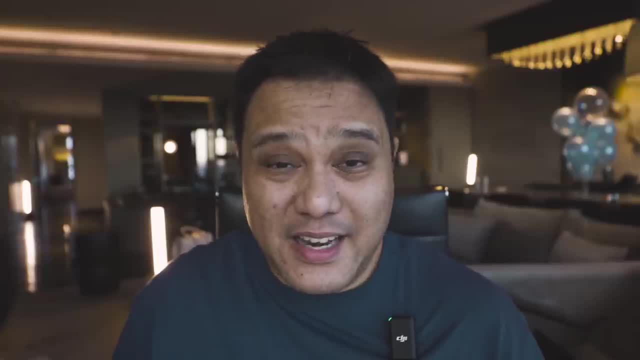 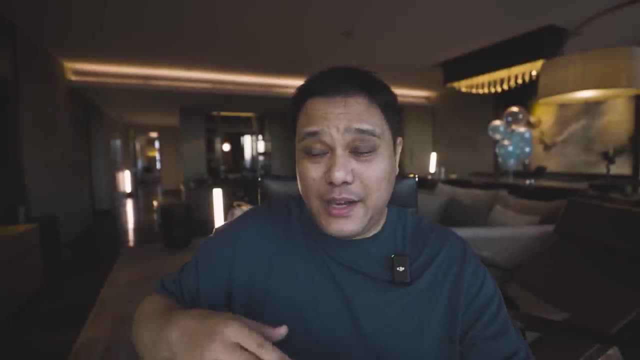 in HTML, which only takes maybe a month, if not less, to understand- Not fully understand, but get a grasp on. And then, why you need to understand is because, now that you understand how HTML works, what is the structure of a body, of a header? You need to know just the basics, enough to be. 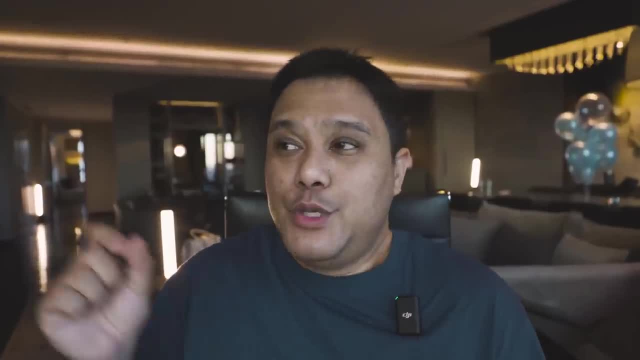 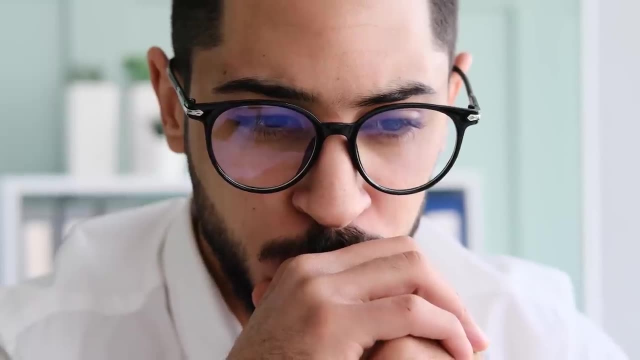 able to use CSS. All right. what's the whole point of using CSS? You use CSS to make things look pretty itself. That is pretty much it. You use CSS to make things more mobile friendly, But people sometimes tend to spend way too much time on CSS when so many 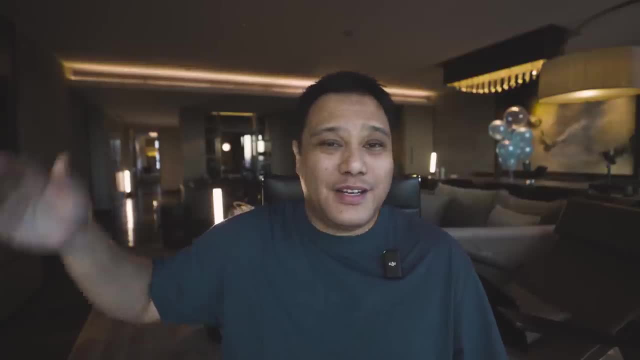 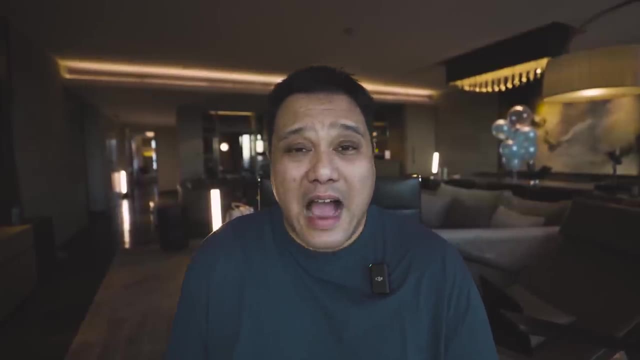 people like me, so many people like Lane, so many people like many other front-end developers tend to use a front-end framework and library to build these beautiful websites. We no longer have to write this from scratch- Well, some companies do, unfortunately- but we use libraries that allow us. 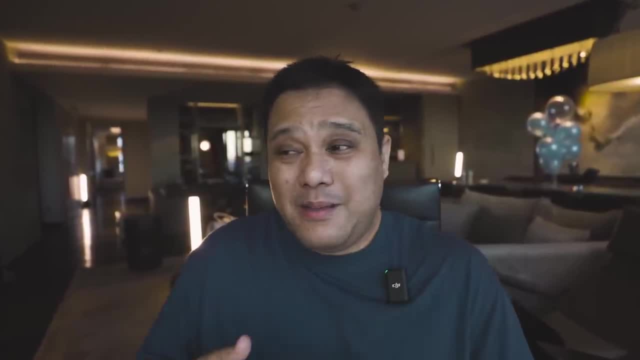 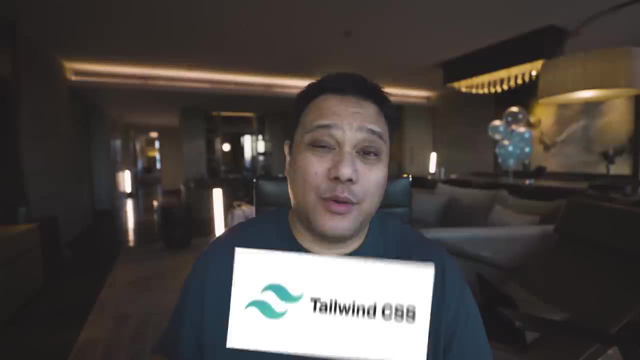 to build these websites more quickly than ever, more fast than ever- And that's why we need to make them as clean as possible by using a CSS or a JavaScript or a front-end library like Tailwind right, Like Tailwind CSS. Now there is one thing I want to disagree with Lane on one point. 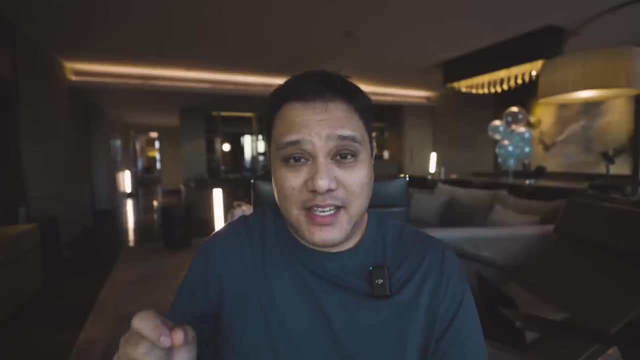 which is this. He did say: HTML in CSS is not the hard part. I agree, but I also disagree. I think that people tend to misunderstand. with Lane primarily being a backend developer. I could also understand why he would say these words, Because as a backend developer- and I now work- as hard as hell. right, What I do in backend is much more difficult than what I've ever done as a front-end developer, right? Maybe it's because as a front-end developer I went to the mid-level position. I never became a senior front-end developer and I moved to backend right after. 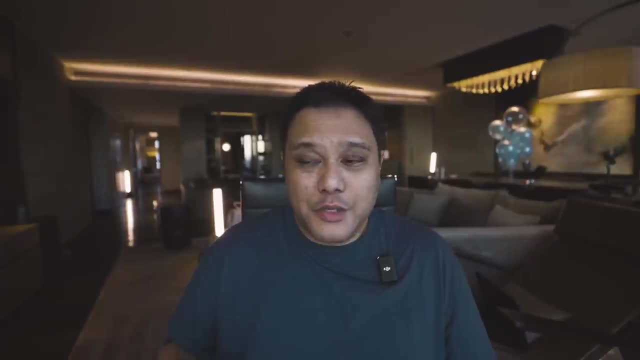 that Maybe that could be it, But from what I've seen, what I do now- backend development- is much more difficult from my perspective. right, But what I'm trying to say is that HTML CSS is a lot harder than what people realize, But what I want people to be able to grasp and understand is that 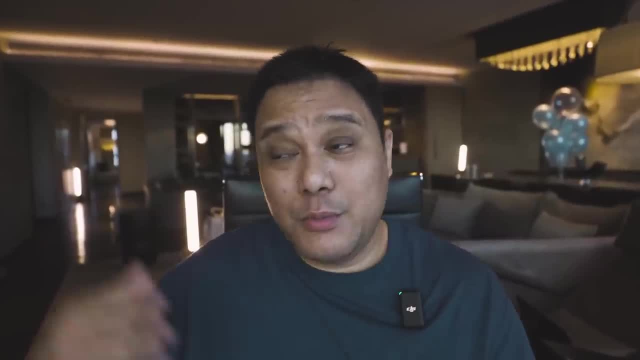 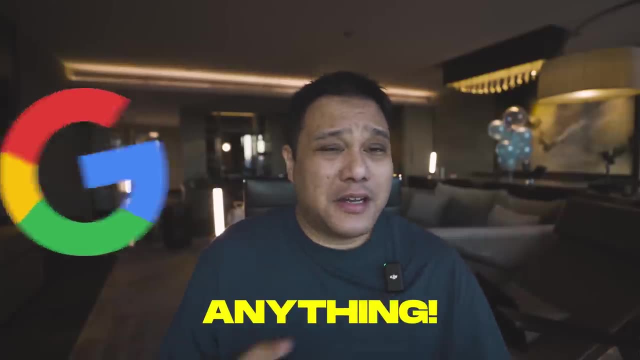 the reason you need to know enough a lot or all of the HTML CSS that's out there before you move on to JavaScript is because of this: Google. You can literally Google anything on how to build anything HTML CSS. You're using a front-end library, a CSS library like Tailwind CSS. What? 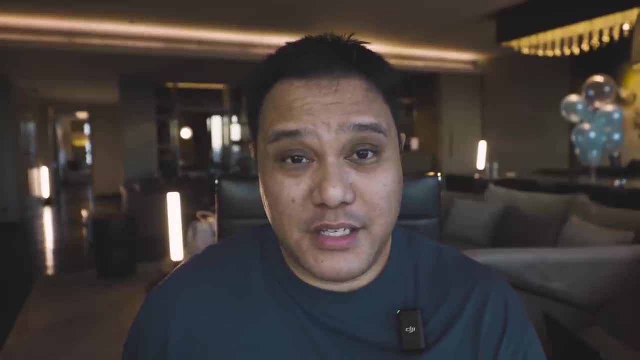 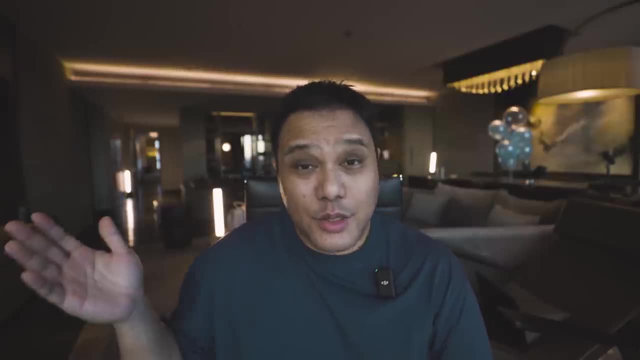 can you do Google? How do I build a hamburger menu using Tailwind CSS? Literally type that into Google. copy the code you find on the internet and paste that into your text editor. Boom, you get a hamburger menu. How do I build a footer using Tailwind CSS or whatever? 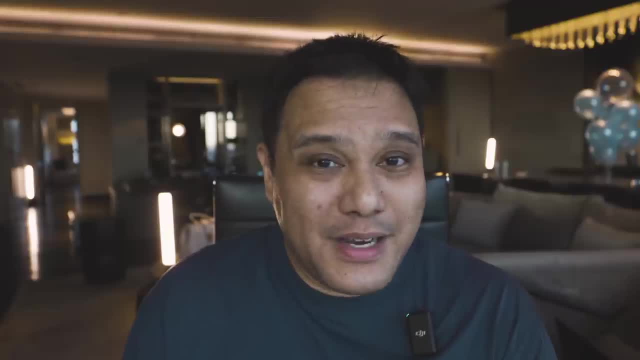 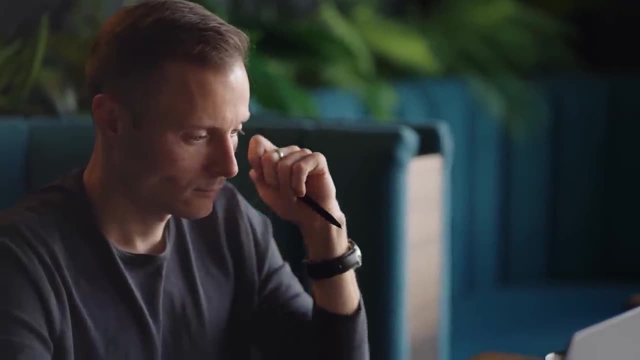 or Bootstrap, you name it. Maybe you're still using Materialize, which has been around for a minute: Google, Google, Google. The whole point of what we're trying to say is that the amount of HTML CSS you need to know is enough to the point where you now know how to Google and research. 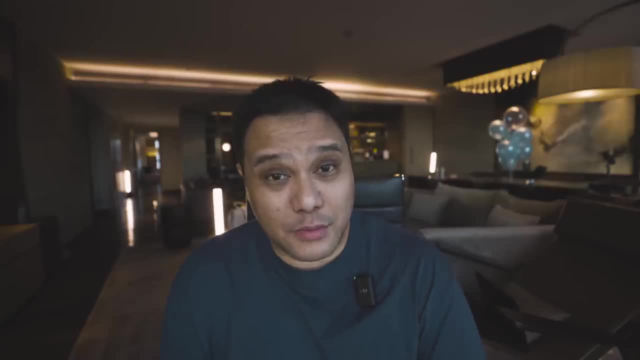 things on the internet to help you build what you don't know as fast as possible. right, That is it. And then what he says next is this: He says that JavaScript is the harder part. I agree with him a million percent on this. 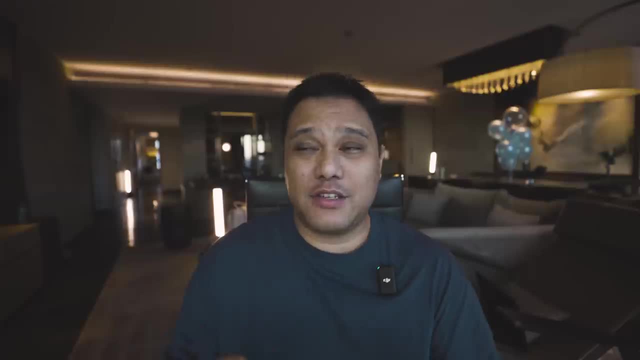 JavaScript will be very difficult for everyone trying to learn how to code. Why? Because JavaScript, for most cases, will be the first programming language that you ever learn. When it comes to JavaScript, it's not even just JavaScript anymore: There's vanilla JavaScript. 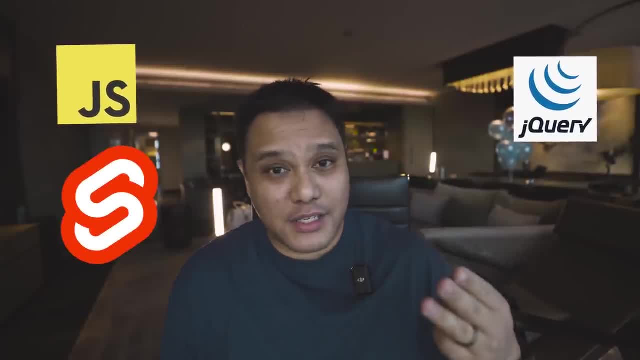 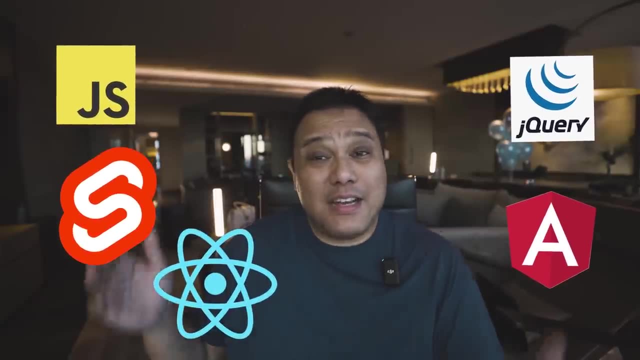 Some companies still use jQuery. right Companies nowadays either use SvelteJS, not as much use AngularJS, but it's still out there. And a lot of other companies now are using ReactJS. And even when you learn ReactJS, that's not even enough anymore. When you learn ReactJS, what is it about? 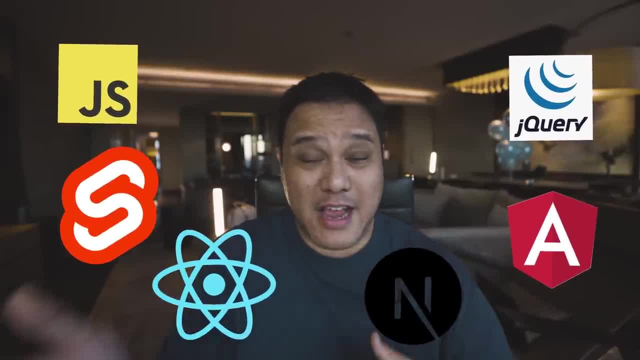 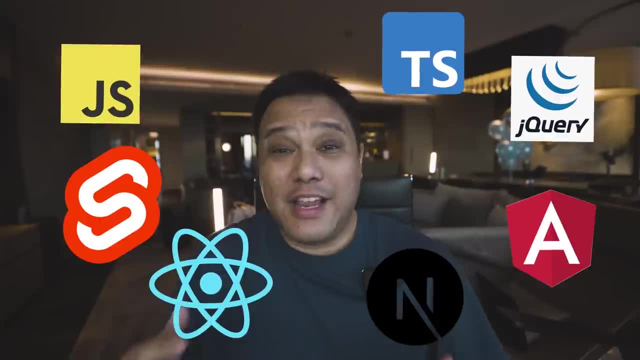 Now you move on to using NextJS. NextJS makes using ReactJS even that much more better. Not even just that, Because you know JavaScript. now you need to use another tool like TypeScript to help you write your JavaScript, to help you write as less bugs and little bugs as possible. 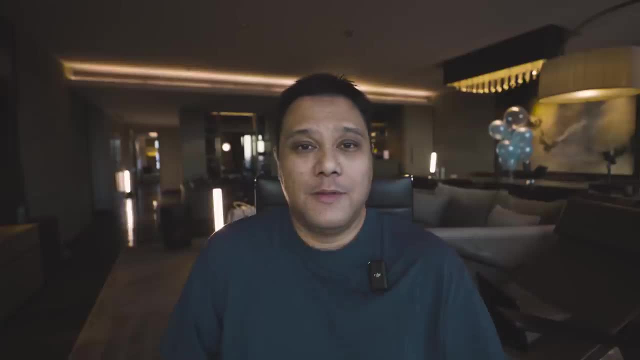 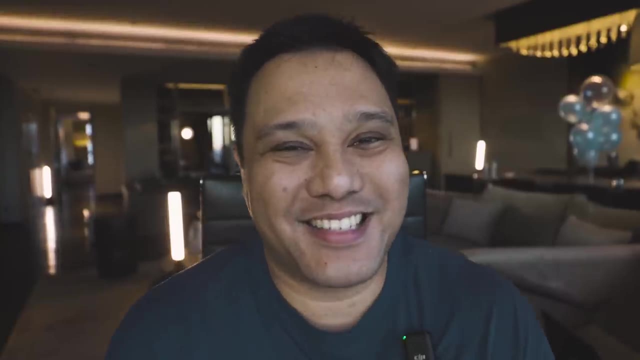 right. So there's a ton more different things that you need to be able to learn. So then, the question then is: how much JavaScript do I need to know? Chris, That I'll talk about next video, Just kidding, Let's talk about that right now. 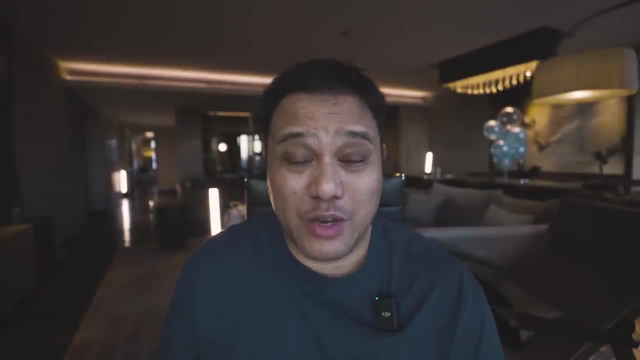 So obviously there are going to be a lot of things that you need to learn in JavaScript- and I can only go over so much- But number one, I think, is the ability to learn JavaScript. So over so much, but number one, i think, the most important part, is to learn the terminology as 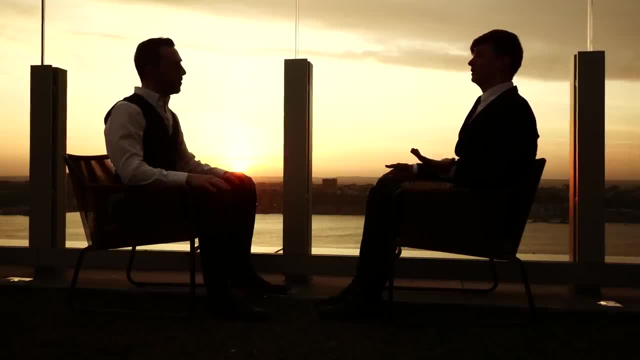 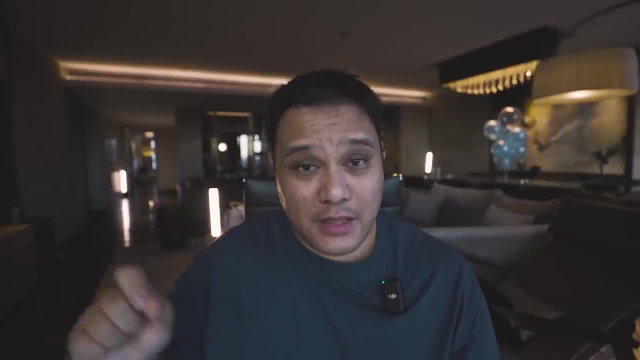 a developer, you need to not just know how to sound like a developer- right, like people say- but you need to know developer talk. why? because when you speak with other developers, especially in javascript, a lot of developers will use terminology that you probably even never heard of, like: what is a map like? how do you map around in the rate? what is an array in the first place? 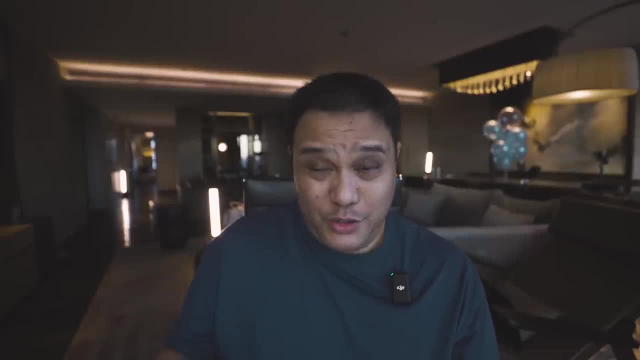 what's an object? what's json? that's not even javascript, but you use json a lot when it comes to javascript. at least i did so- being able to understand these different terminologies- functions to for loops, to you name it. just being able to understand the terminology on different. 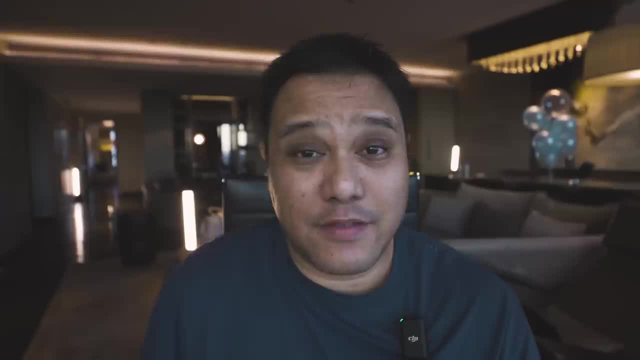 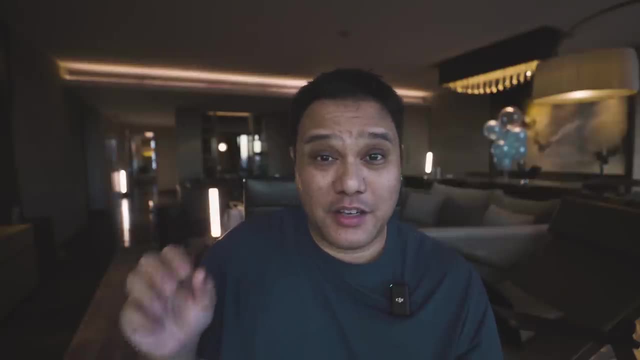 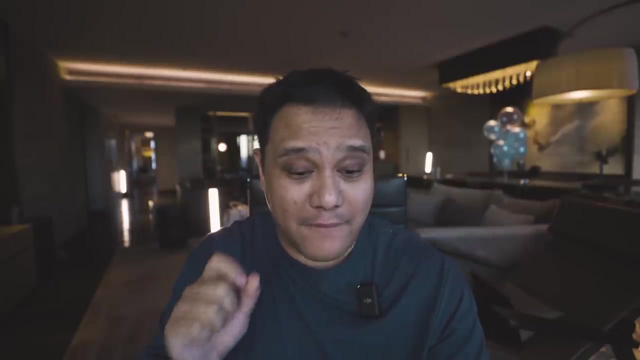 things is extremely important when you start learning javascript. don't just skip around things when javascript understand the terminology. now in the link description below, i'll put a list of different terminology that you can learn when it comes to javascript. hopefully this helps, but let's go to the next part. all right, so i'm gonna go through this list really quick on my phone. all. 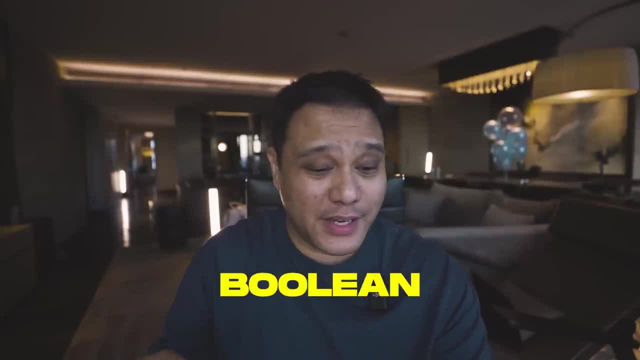 right, so number one when it comes to javascript. you need to learn things like your boolean. you need to learn number strings, etc. the different operators when it comes to working with javascript. right, you need to learn even typescript, to help you again avoid running bugs. typescript will save. 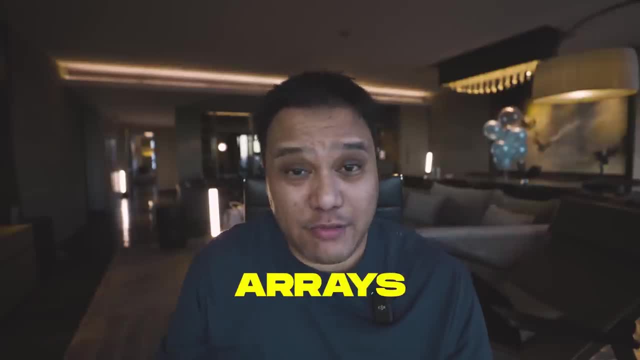 your life as you learn this. next, what you need to learn are things like how to work with arrays, how to work with different objects, what the hell is even object oriented programming? the basics are what you need to learn when it comes to this, and then and then, even on top of that, you need to 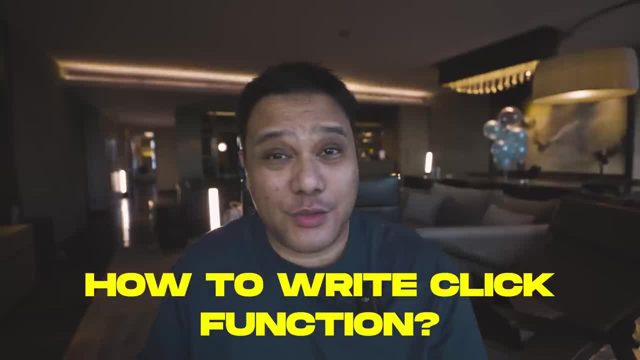 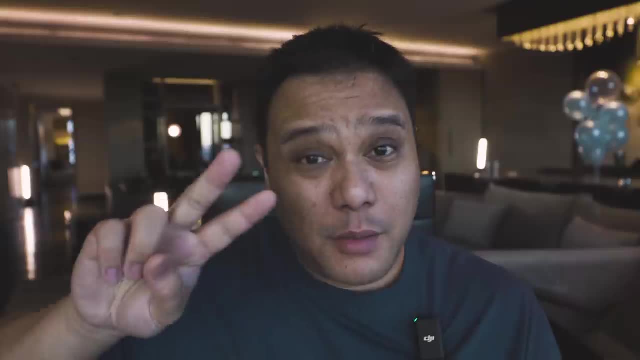 learn how to manipulate the dom. how do you write click functions? when it comes to javascript, what is a map? what is a function? what is the fl statement? how to write the fl statement. how to use operators like double uh equal sign or triple equal sign. when to use 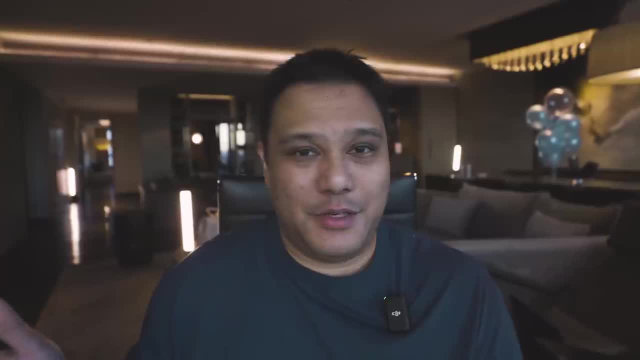 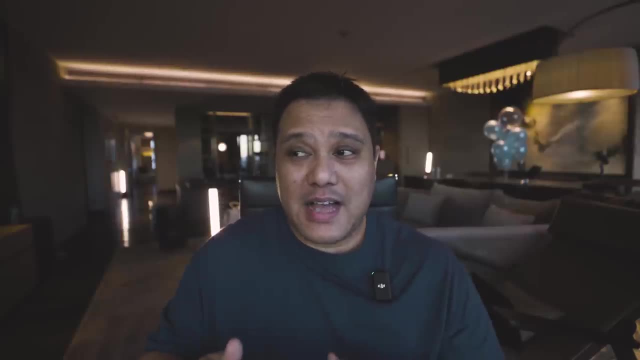 back ticks. when to use semicolon. yes, you don't even really. you only really need to use semicolons in javascript, but pretty much all of the basics when it comes to javascript- enough to allow you to manipulate the dom. on top of that, you need to learn about events listeners. when to wait for a.